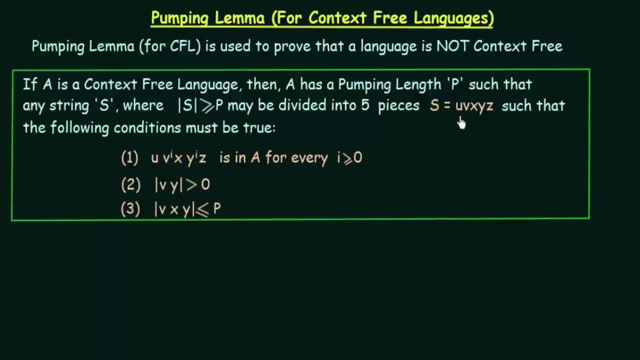 that string S can be divided into 5 pieces, such that S is equal to u, v, x, y and z. So if you remember, when we studied for pumping lemma for regular languages we divided the string into three pieces. But in this pumping lemma for context, free language, we will divide the string into five pieces: u, v, x, y and z, such that the following conditions must be true: 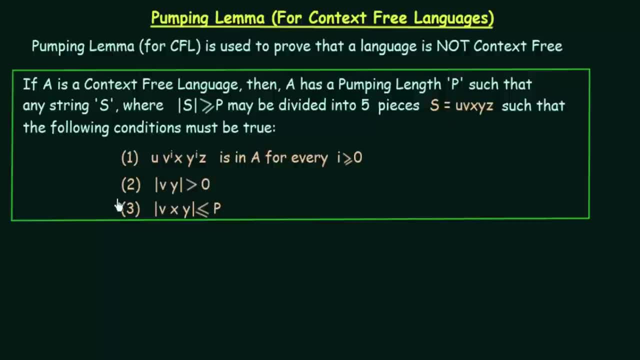 So if you divide it into five pieces like this, these three conditions must be true. And what are they? u. v raised to i. x. y raised to i. z is in: A for every i greater than or equal to 0.. 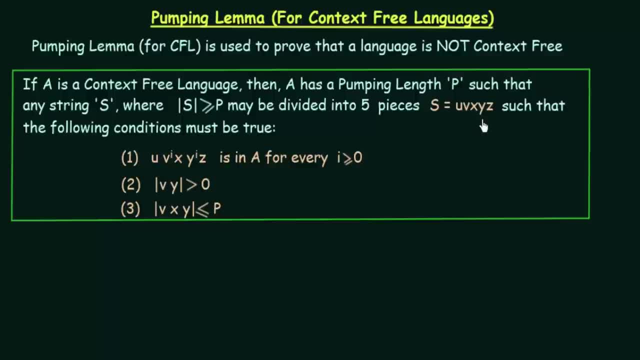 So you have divided s into u, v, x, y and z, And here if you raise v to the power of i and y to the power of i, where i is greater than or equal to 0, then the string that you get, even after doing this, should also be equal. 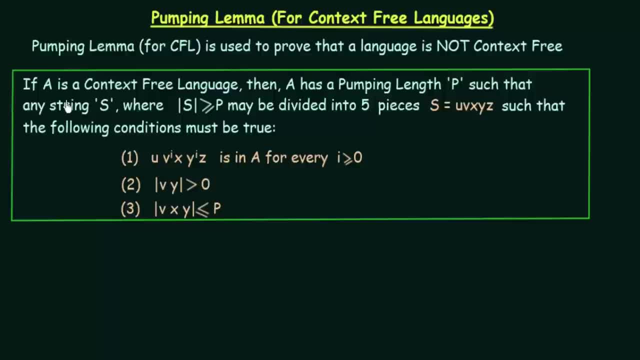 In A. that means that string also should belong to the language A. And the second condition says that the length of v and y should be greater than 0.. And then the third condition says that the length of v, x and y should be less than or equal to p, which is our pumping length. 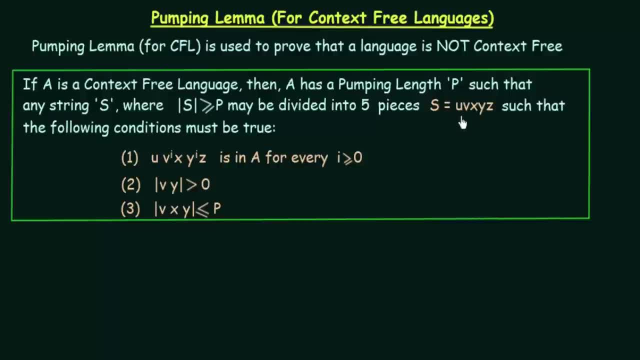 So remember that this u, v, x, y, z- they are not strings, but they are the parts into which you have divided the string s And after you divide this, these three conditions must be true, And if these three conditions are true, then we can say that it is a context-free language. 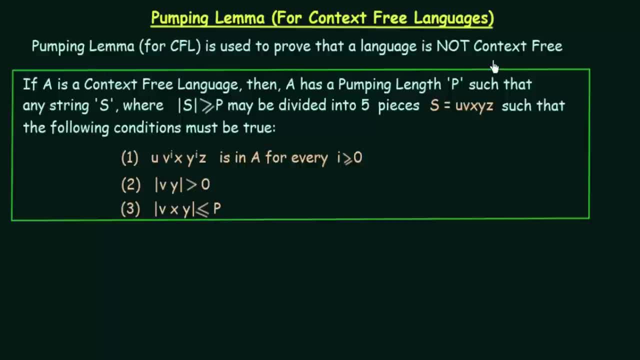 So we are going to prove that a language is not context-free using this pumping lemma. So this is the conditions that we know and let's see how we can prove it using pumping lemma. So, in order to prove that a language is not context-free, using pumping lemma for context-free languages. 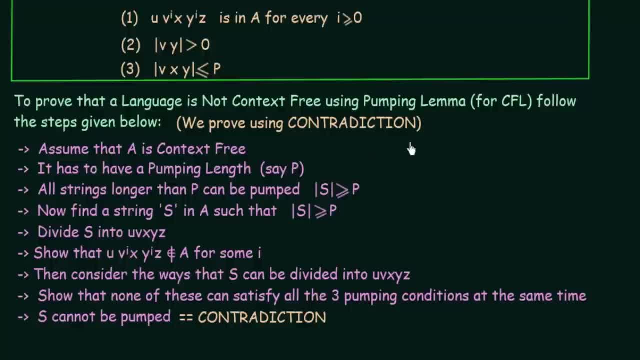 we have to follow the steps that are given below. So, just as As we did in the case of pumping lemma for regular languages, even in this case we will prove it using contradiction, Alright, so here we have the three conditions given, and we already defined them. 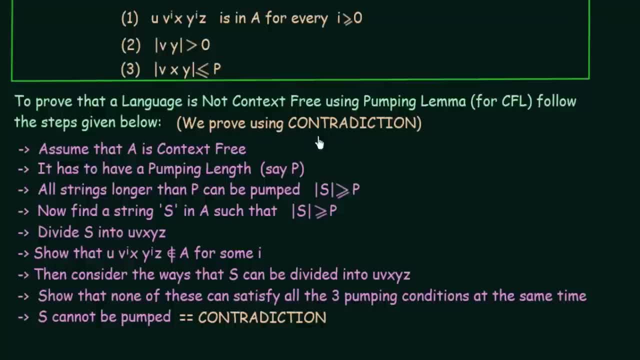 And now, since we are going to prove it using contradiction, what we will do is we will assume that a is context-free. So we have a language that we call a and we will assume that it is context-free for the beginning. So we have already read that if a language is context-free, 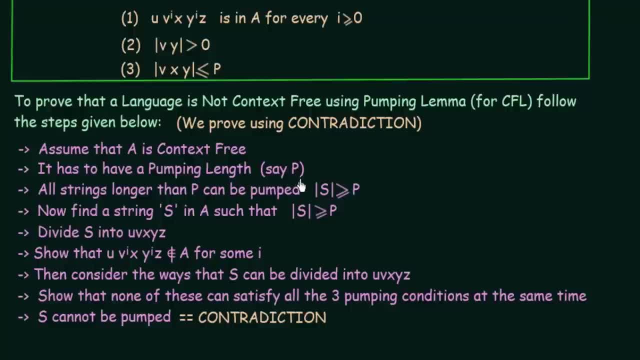 Then it has to have a pumping length, and let's call it p. So, as we assumed, a is context-free, so it should have a pumping length, which we will call p, And then all the strings longer than p can be pumped. So any string whose length is greater than or equal to p can be pumped. 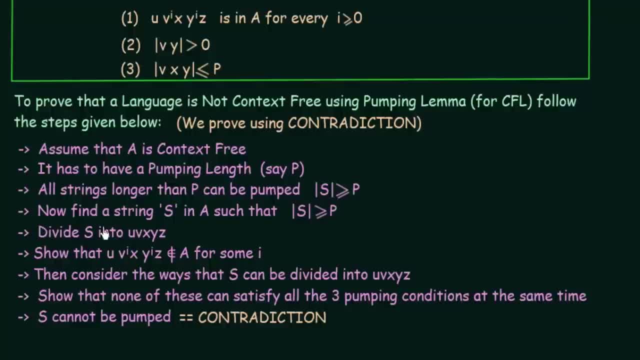 That's what we read above. Now what we will do is we will find a string s in a such that the length of s is greater than or equal to p. So we have our language a, and from this language a we will take a string which we will call. 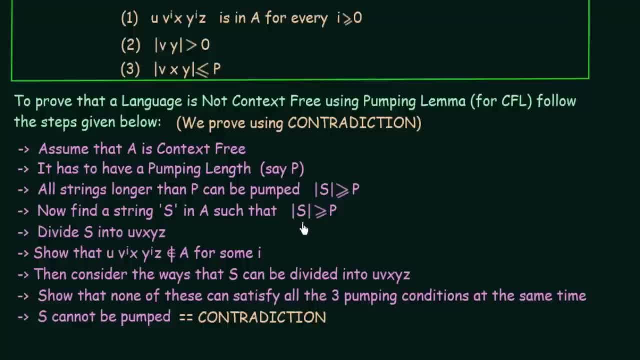 s such that the length of this string s should be greater than or equal to P, which is our pumping length. now, after you take that string, as we will divide that s into five parts: u, V, X, Y and Z. so we have a string and it is divided into. 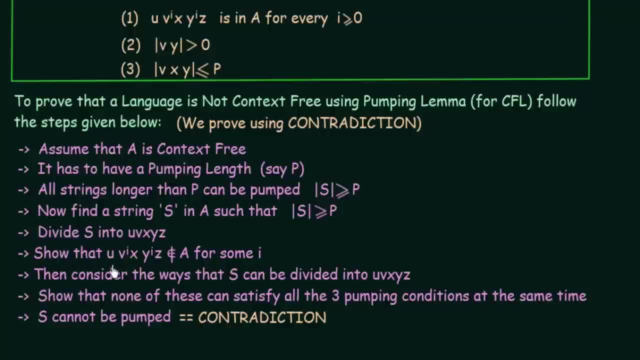 five parts now. now we will show that u, V raised to I X, Y raised to I Z does not belong to a for some value of I. so you have divided this s into these many parts. so when it is divided in this way, it is lying in this language, a we know. 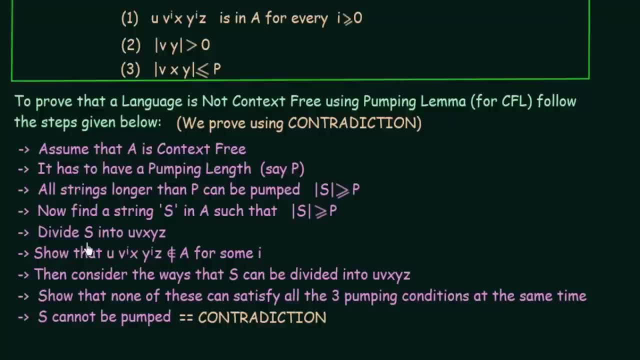 that now we will show that this string s, which you have divided into this five parts, this part of V, you have divided into this many parts. so when it is divided in this way, it is. and this part of Y, when you raise it to some power of I, that means, if you 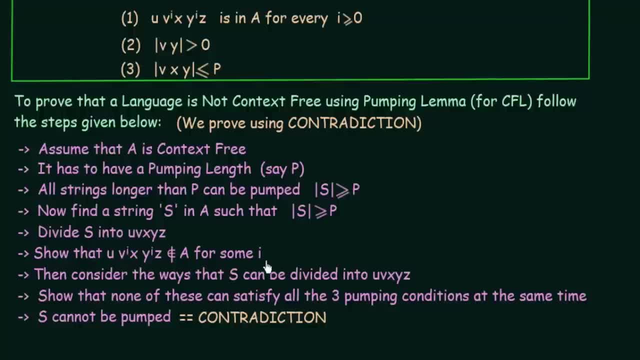 repeat this V part and Y part some- I number of times. this new string that you obtain, you have to show that it does not belong to the language a. so we don't know what is the language right now, but when you have the example you will know. 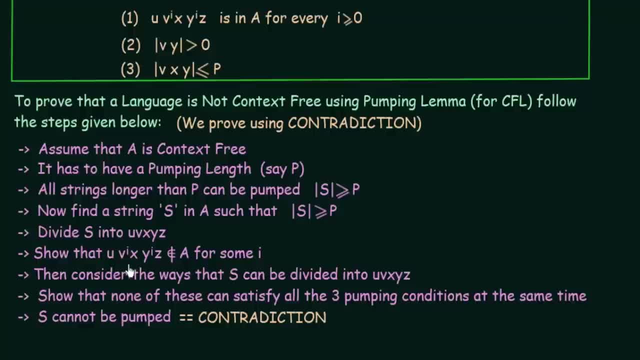 some rules that have to be followed for the language. so once you divide it in this way and raise it to this powers, you have to show that it does not belong to this language. a. after that, consider the ways that s can be divided into: UV, X, Y.